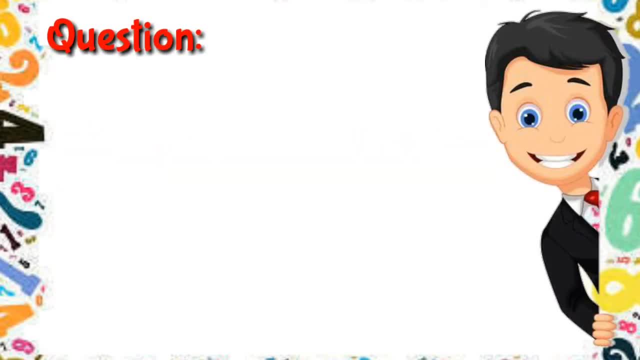 What's up, kids, I have a question for you. Do you always keep your things organized or in order? Great, Why so? It keeps your area clean and helps you find things easily right. And today you will be needing your skills in arranging things as we learn. 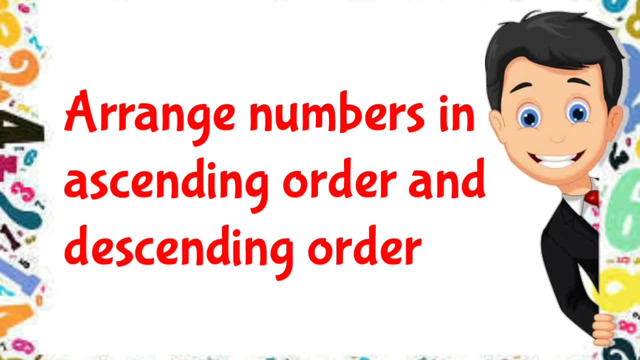 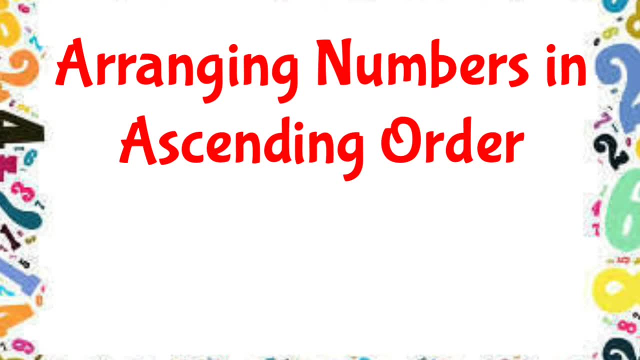 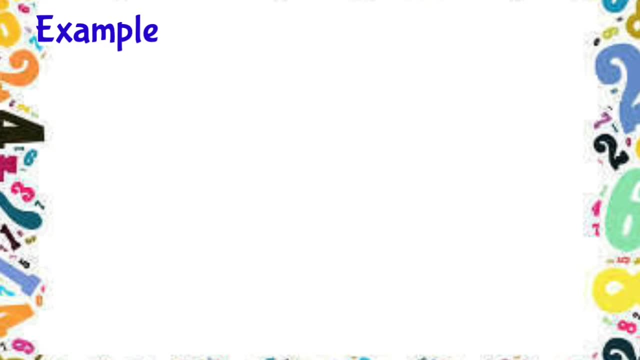 how to arrange numbers in ascending and descending order. So let's get started. Let's have arranging numbers in ascending order, first meaning from the smallest to the largest number. For example, if we arrange 58,, 327,, 145, and 89 in ascending order, 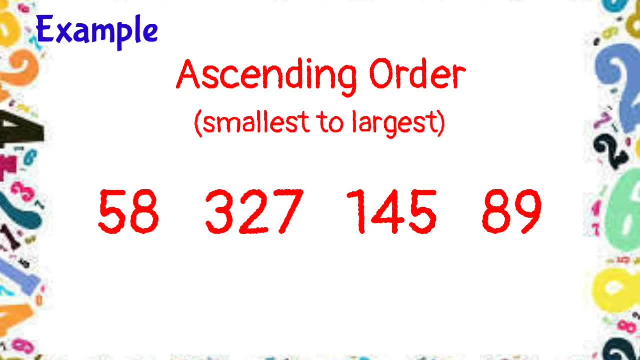 or from the smallest to the largest number. the order should be 58,, 89,, 145, and 327.. Another example: Arrange 1,907,, 245,, 6,879, and 134 in ascending order. The first number should be the smallest one, which is 134,, to be followed by 245, then 1,907, and. 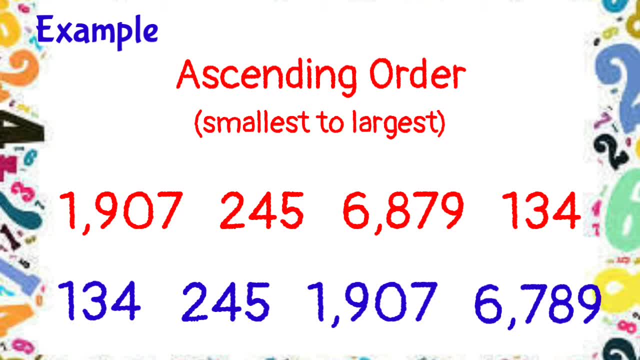 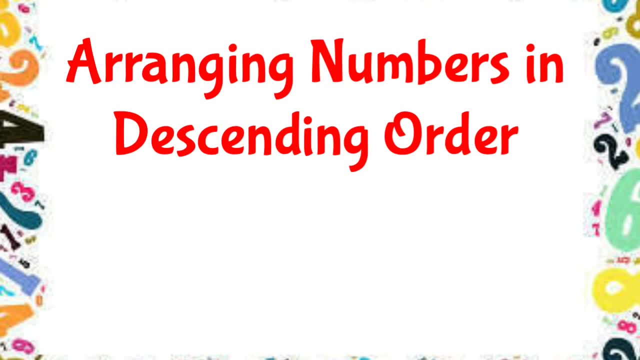 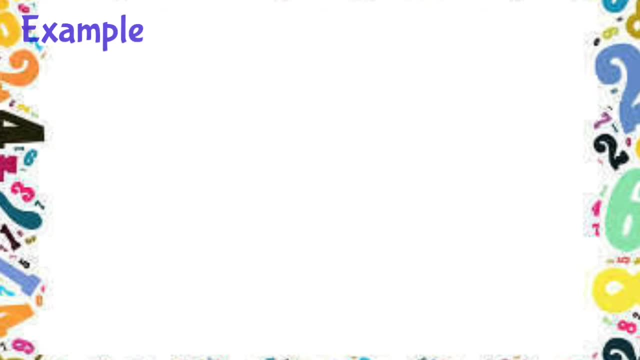 6,789, being the largest number in ascending order. Now let's move on to arranging numbers in descending order, or from the largest to the smallest number. It is simply the opposite of ascending. For example, if you arrange 698,, 107,. 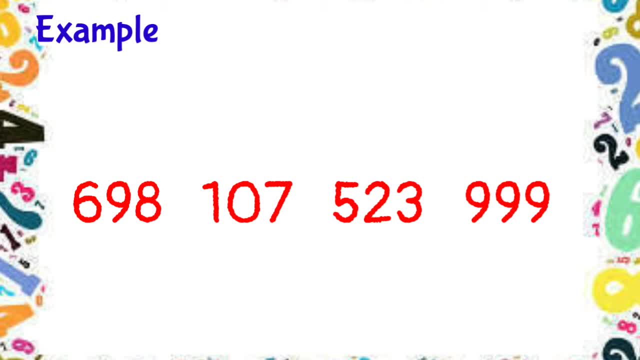 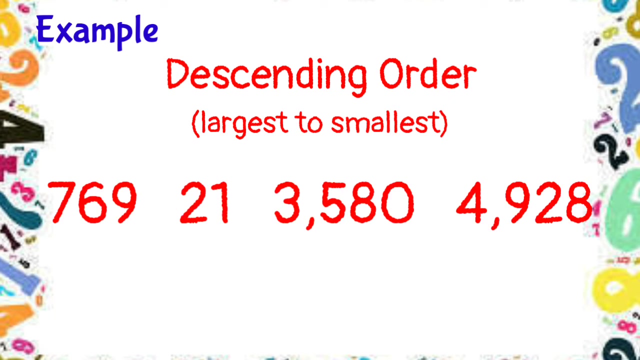 523, and 999. in descending order, the sequence should be from the largest to the smallest number, so the first number should be 999, to be followed by 698, then 523, and 107.. Another example: Arrange the following numbers in descending order: 769,, 21,, 3,580, 4,928.. The correct order is: 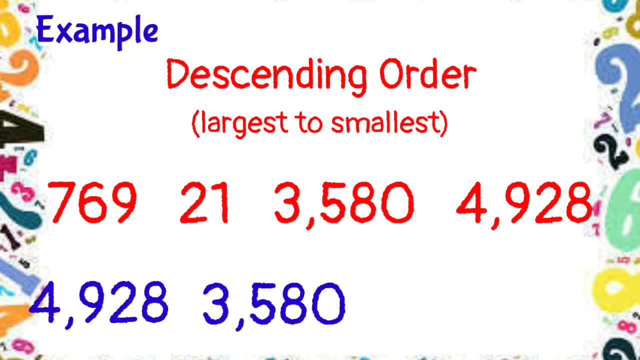 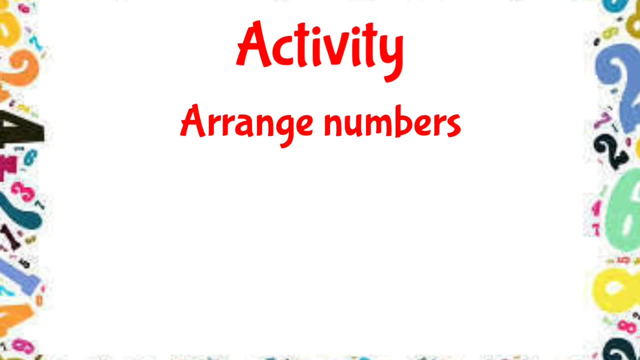 4,928,, 3,580,, 769, and 21.. Is it understood? Then let us have an activity. Your task is to arrange the following numbers in ascending order for the first part and descending order for the second part. Let's have part 1.. Arrange the. 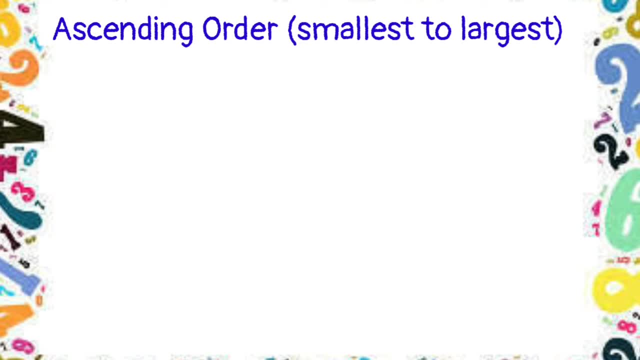 following numbers, in descending order or from the smallest to the largest number: Number 1.. 51,, 32,, 98,, 74.. Let's answer. The order should be 32,, 51,, 74, and 98.. Number 2. 591, 234,. 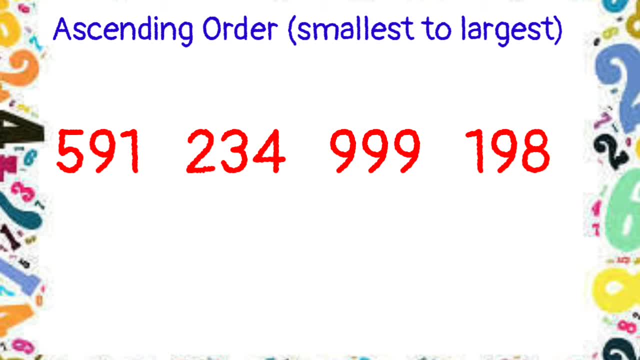 роп 234.. 999, and 198.. The sequence should be spiders 17- 17.. The order should end on the highest point. Then G must not be durant 124.. Then you must còn at the top of the last number. 131.. Then G must not be during 14.. Then you must read theutr chamber, per folio, neutrinos 291.. Then the order comes to the last button. Ungreditably, you can reach the name of priority. 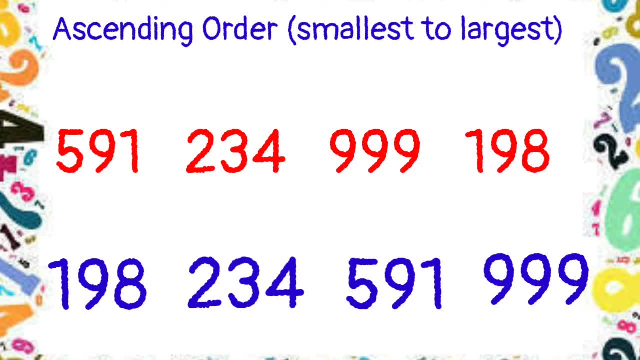 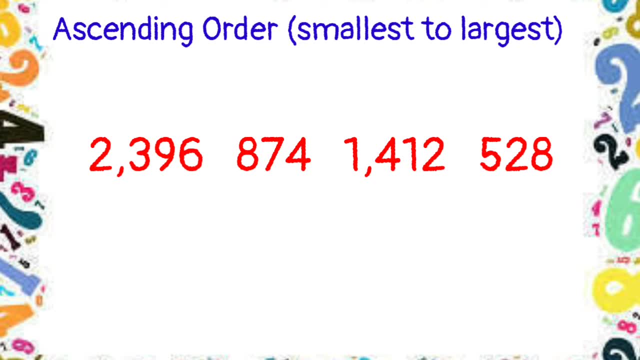 www.kiscoopb.com And let's come to the order 3. Number today, we're using a sounding order R with a stressed C. � 528. The correct order is 528, 874, 1,412, and 2,396. Number four, 1,890, 1,234, 1,567, 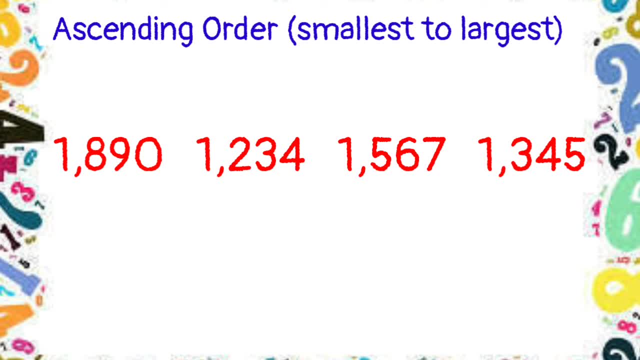 and 1,345.. So from the smallest number, 1,234,, then 1,345,, next 1,567, and the largest number 1,890.. Number five: 57,, 5,301, 10,239.. The sequence should be: 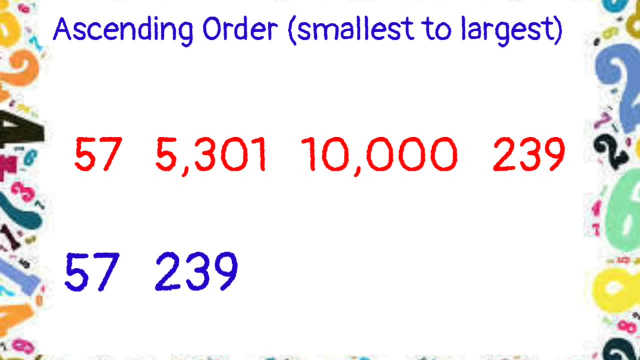 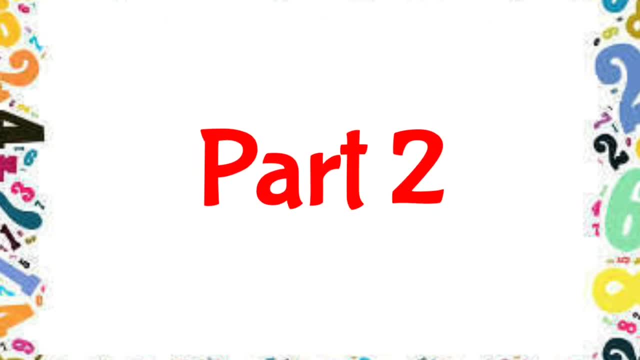 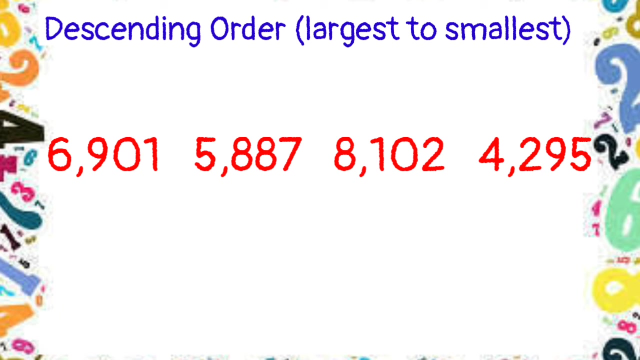 57,, 239,, 5,301, and 10,000.. Now let's move on to part two. Arrange the following numbers in descending order or from the largest to the smallest. number Number one: 6,901,, 5,887,, 8,102, and 4,295. 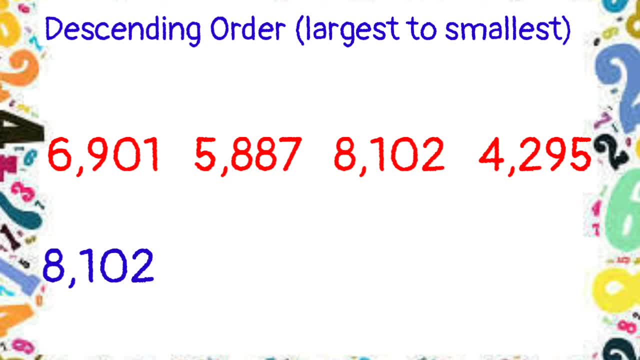 So the sequence should be 8,102, 6,901,, 5,887, and 4,295.. Number two: 980, 890, 809, 908.. The order should be 980, 908, 890,. 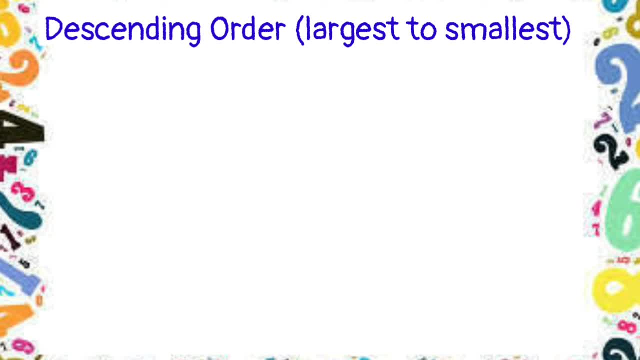 and 809.. Number 3, 910,, 1078,, 2,195, and 3,412.. Let's answer 3,412,, 2,195,, 1,078, and 910.. Number four: 1,218,, 1,278, and 1,809.. The order should be 1,790, 809, 908.. 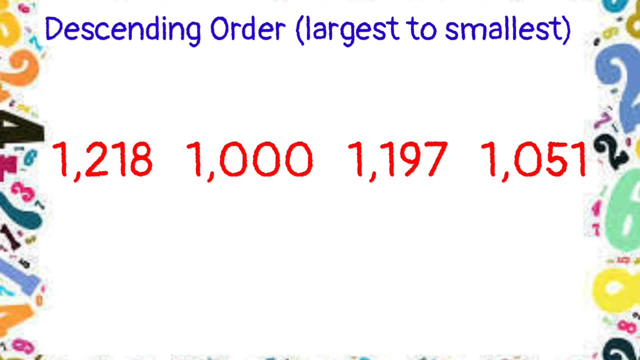 So the sequence should be 980, 909, 809, 908.. The order should be 980,, 908,, 880, and 910.. 1,000,, 1,197, and 1,051.. 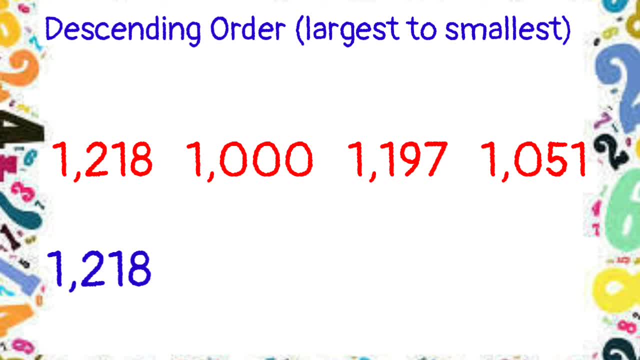 The correct order is 1,218,, 1,197,, 1,051, and 1,000.. Number 5. 345, 3,405,, 35, 3,450.. Alright, let's answer. 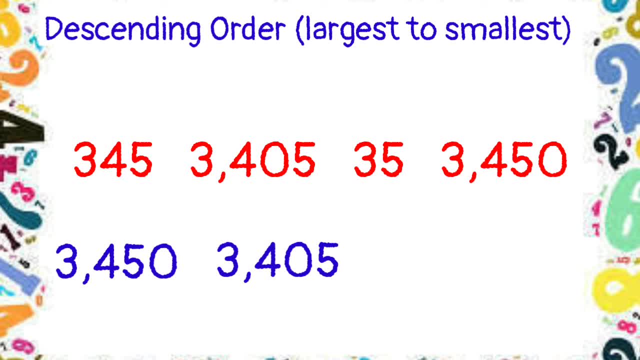 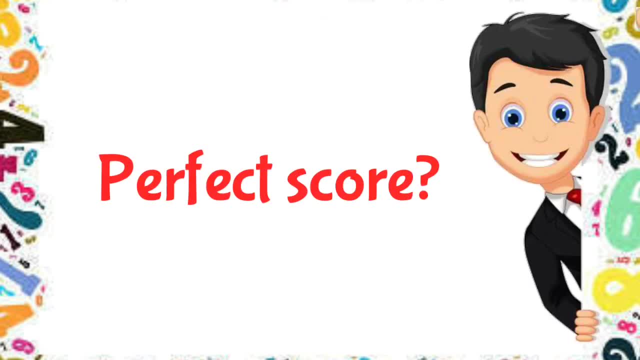 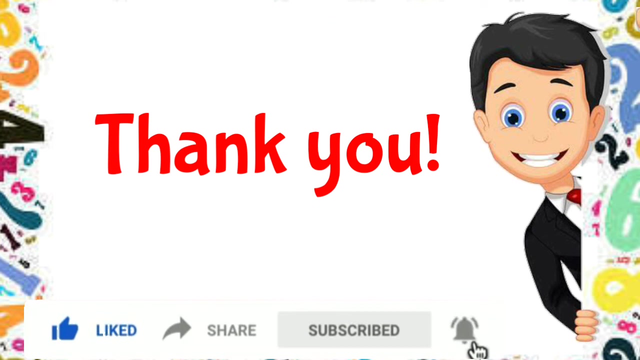 3,450,, 3,405,, 345, and 35.. So did you get the perfect score? I just hope that this video has helped you improve your skills in arranging numbers, be it in ascending or descending order. Thank you for watching this video, kids. Bye. Subtitles by the Amaraorg community.